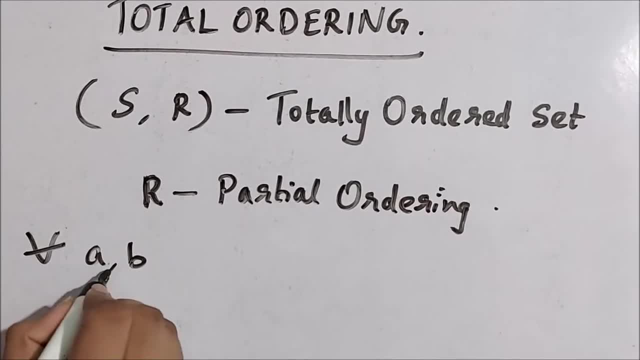 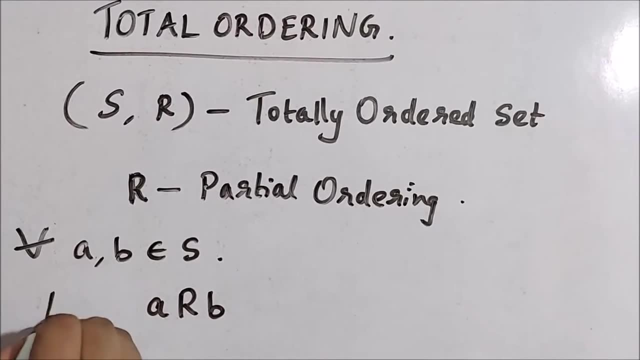 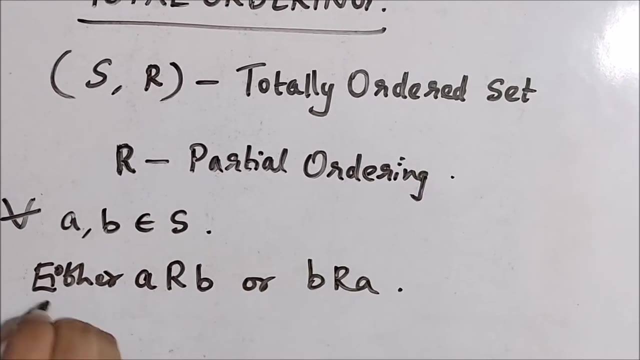 A. So for all of the pairs- A- B- belonging to the set S: Okay, Either A should be related to B. Okay, Either A should be related to B or B should be related to A. In other words, if you take any pairs belonging to the set S, they should be comparable. 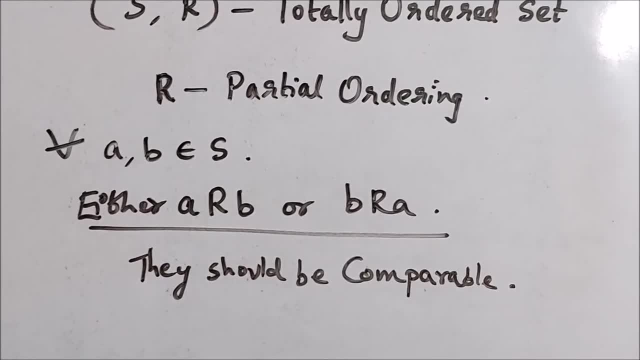 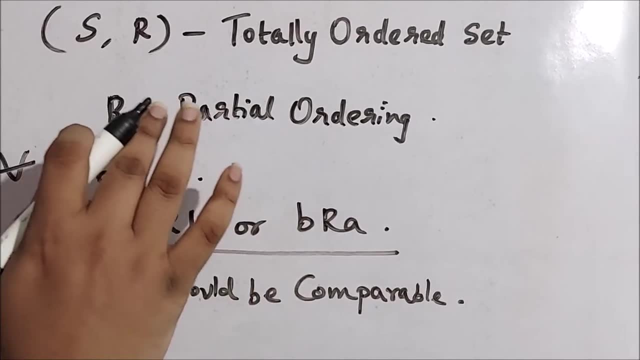 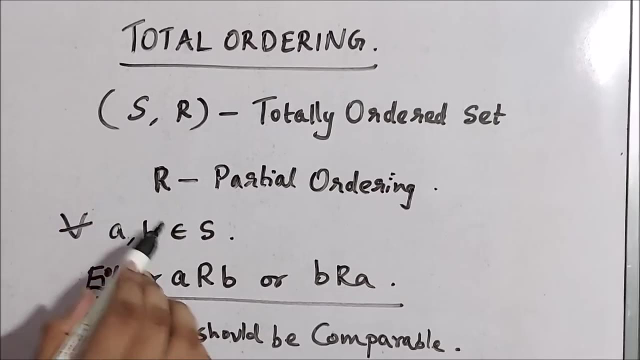 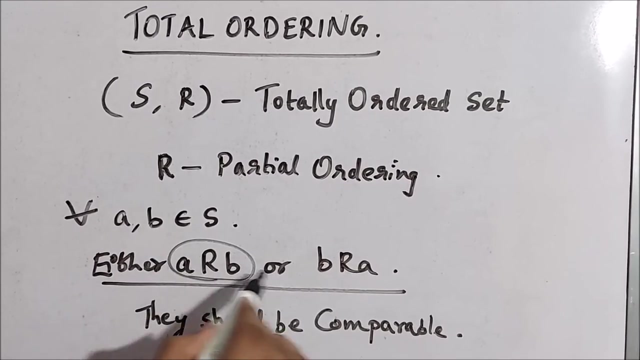 Okay, Now you the first of all, for a relation R to be a total ordering relation, R has to be a partial ordering relation, meaning that R has to be reflexive, antisymmetric and transitive. Also, the relation R which is defined on the set S. you take any two elements, A and B, belonging to the set S. Either A should be related to B or B should be related to A. So that is what means comparable, Okay. 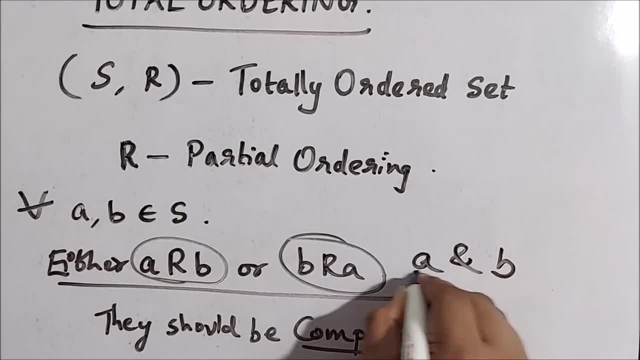 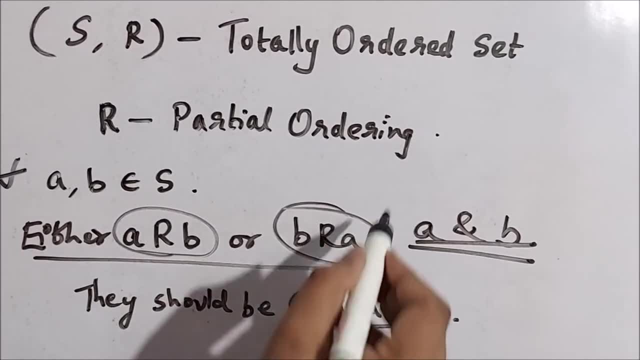 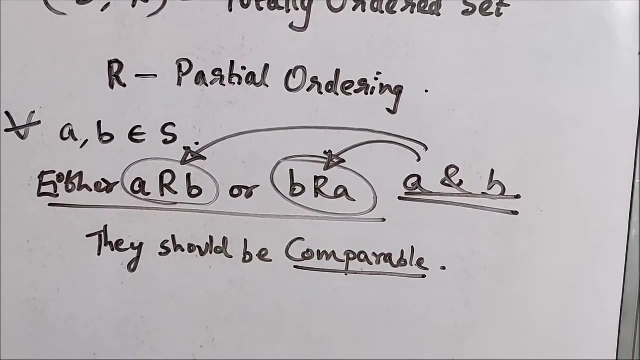 Okay. In other words, A and B are comparable means that when we say two elements, A and B, are comparable with respect to the relation R, it means that either A is related to B or B is related to A. If both are not there, then that means that A and B are incomparable. 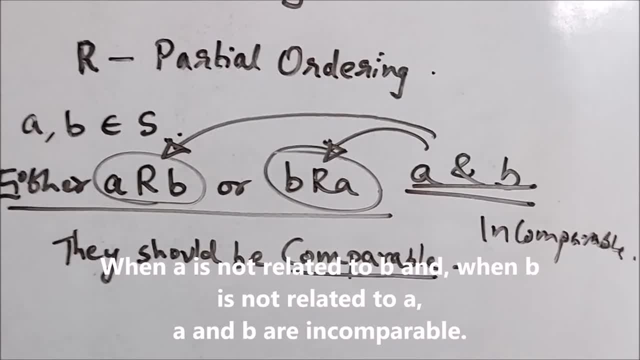 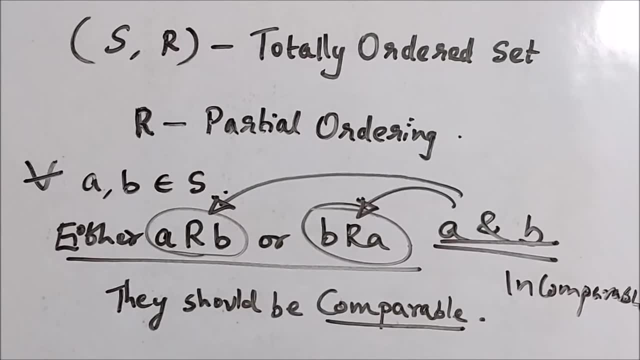 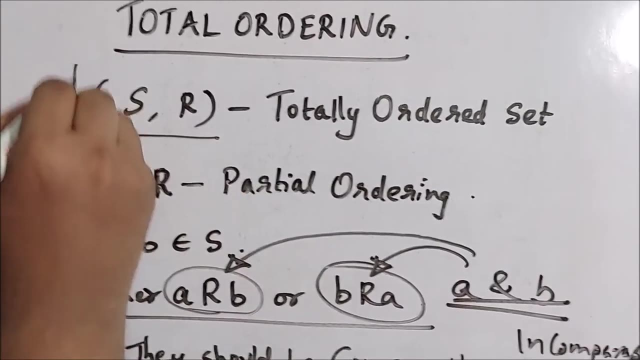 Okay. So for a relation R to be a total ordering it has to be a partial ordering And if you take the set S, You take any two elements belonging to the set S. it has to be the case that A is related to B or B is related to A. Then the set S, together with the relation R, is called the totally ordered set. Okay, 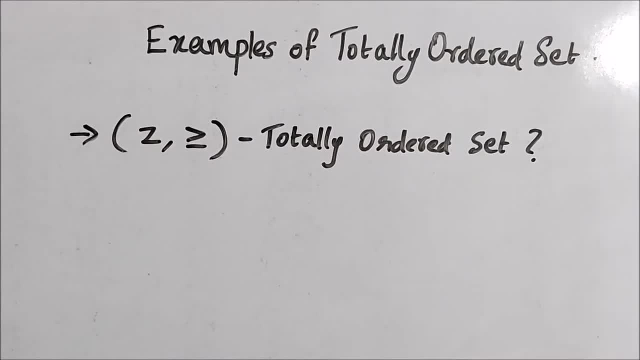 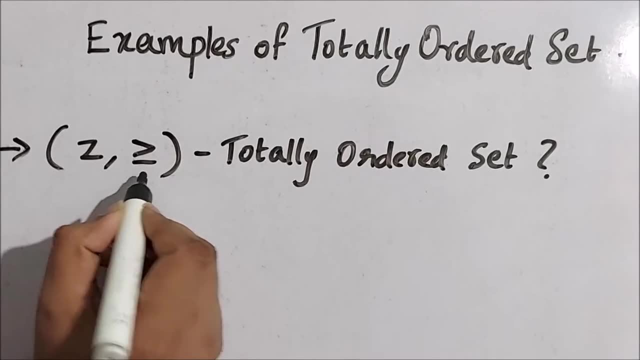 Okay. So let us see some examples of totally ordered set. Right, So given Okay The set of integers together with the greater than or equal to relation. whether that is a totally ordered set or not, that is a question, Okay. 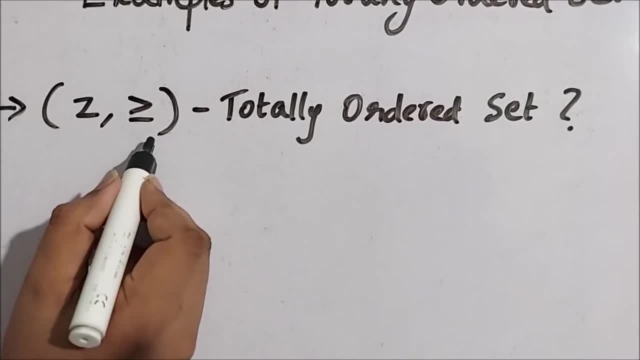 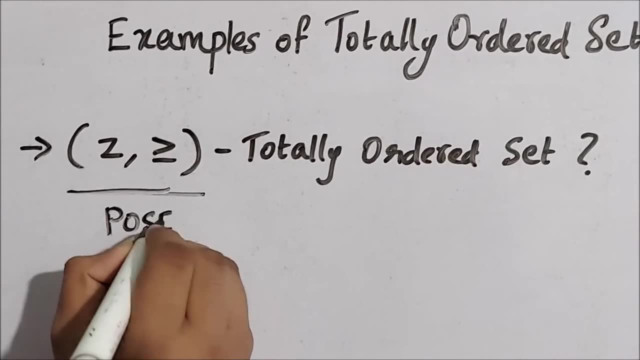 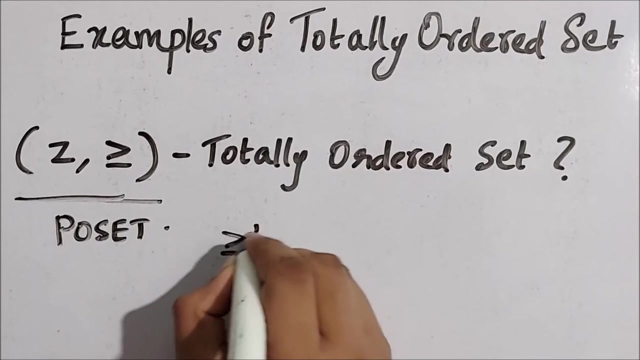 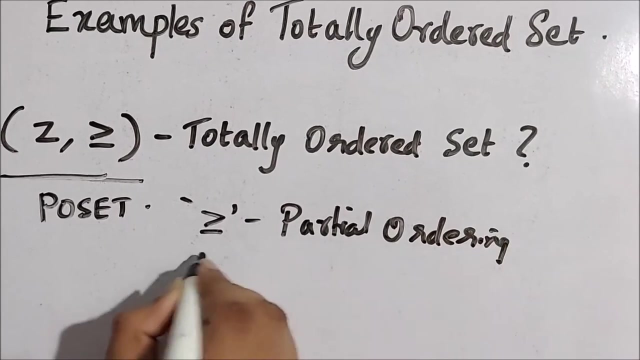 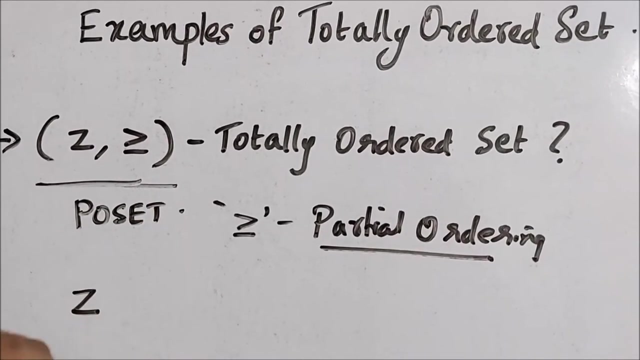 Okay, So we have seen this, Which is an example of a partially ordered set. I mean, we have already discussed that set comma greater than or equal to is a partially ordered set. Right, We have proved that Now. Okay, So one condition is met: that the greater than or equal to relation is a partial ordering relation. Right, That is, That was one condition for the greater than or equal to relation to be a total ordering. This is a partial ordering. Now you consider the set of integers, The set. 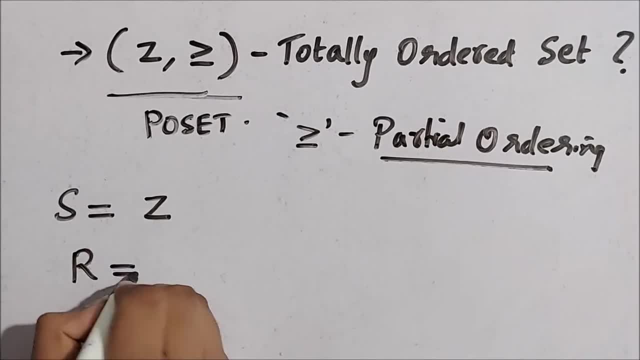 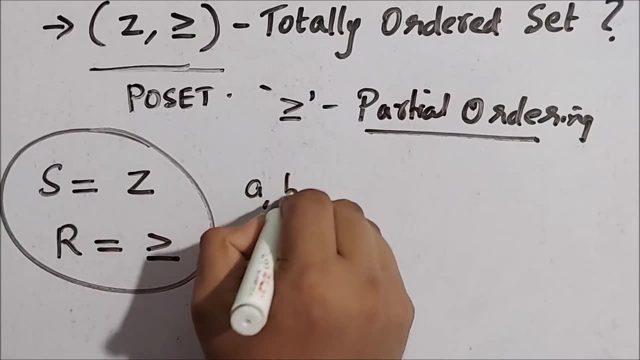 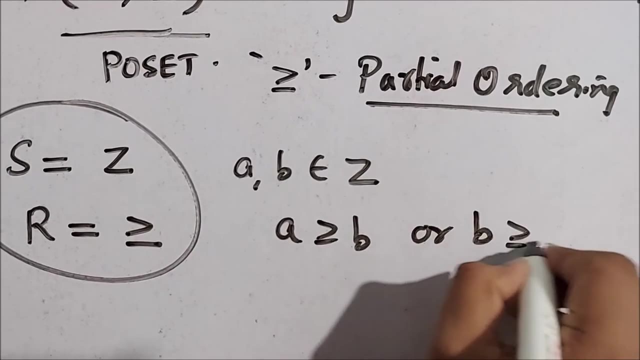 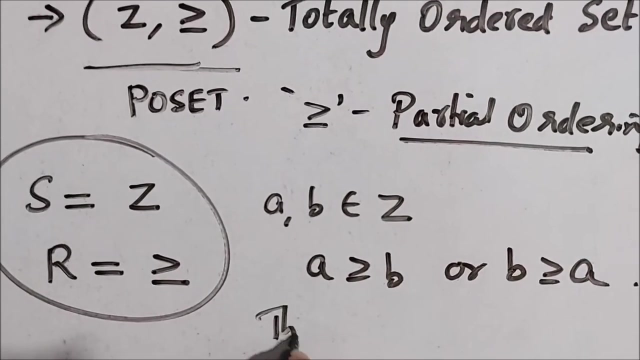 S. Here is a set of integers and the set, The relation R, is a greater than or equal to relation. Okay, This is the case here. Now you take any two elements- A, comma, B- belonging to the set of integers. A is at least B or B is at least A, Meaning that you take any two elements belonging to the set of integers. They are comparable, Right. 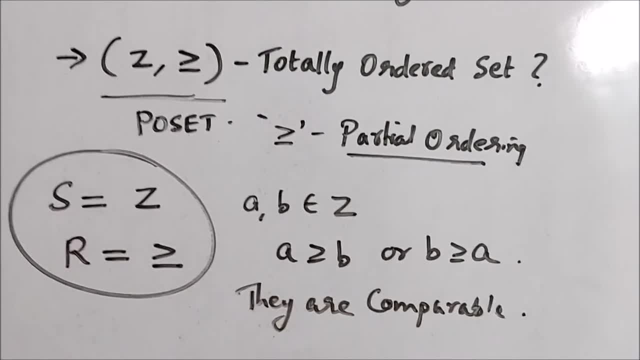 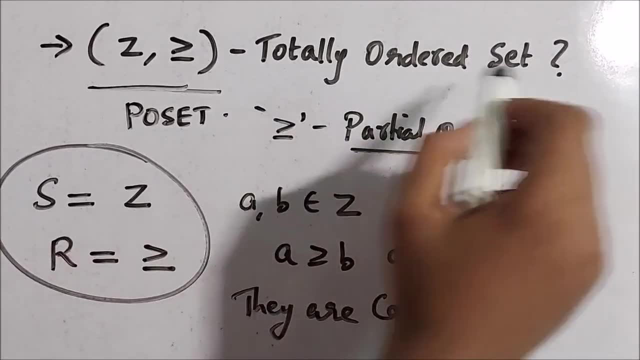 So either A is related to B or B is related to A when the relation is greater than or equal to, and the set is a set of integers. So set comma greater than or equal to is a totally ordered set. So this is a totally ordered set. This is an example for a totally ordered set. 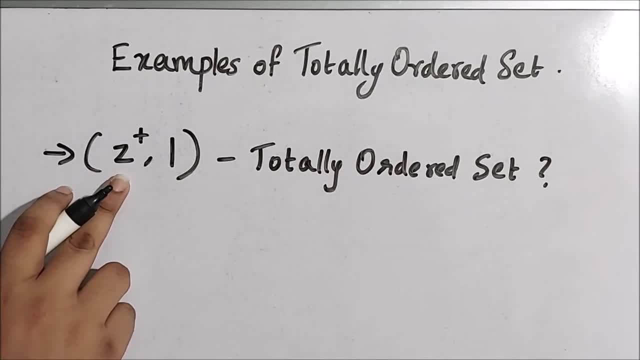 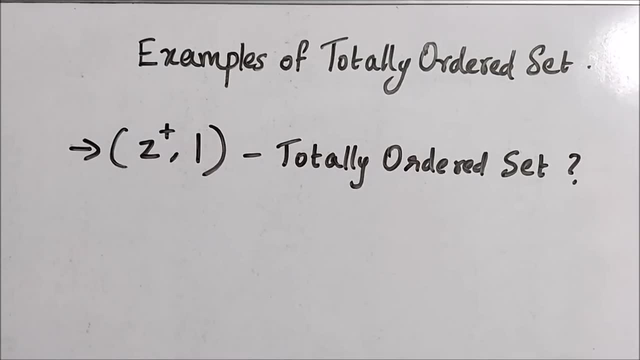 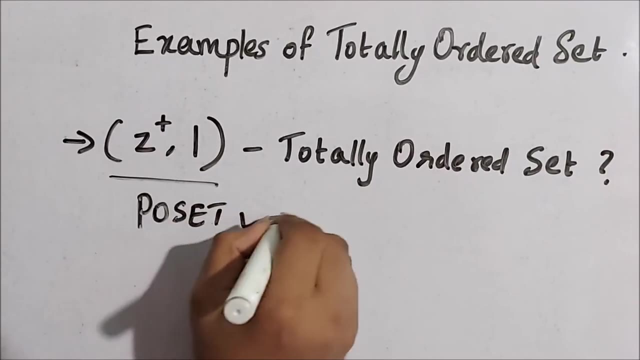 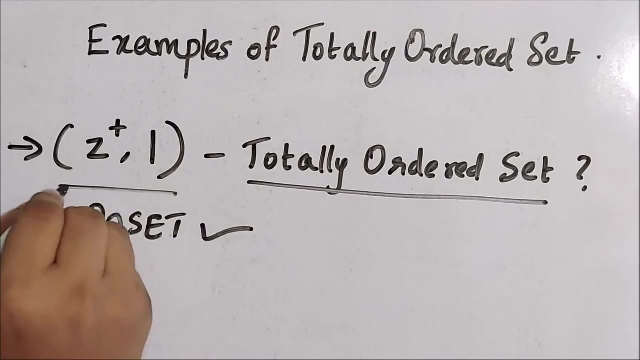 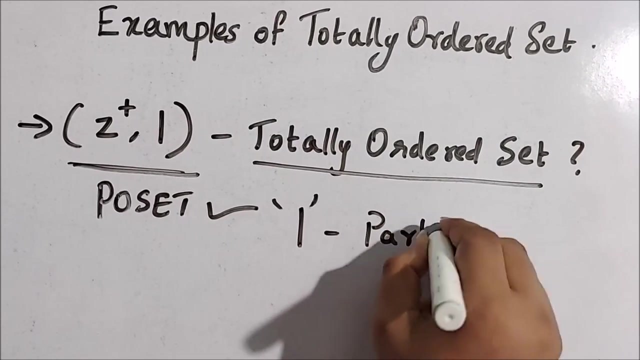 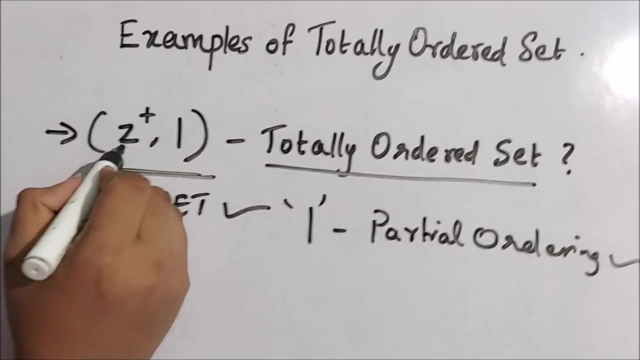 So now the question is whether the set of positive integers, together with the divides relation, whether it is a totally ordered set or not. We have seen that we have proved that the set of positive integers, together with the divides Relation, This is a partially ordered set, Right. We have proved that. Now the question is whether that is a totally ordered set or not. So obviously the divide- as since we have proved that this is a posit or partially ordered set, The divides relation was a partially ordering relation Right- Was partial ordering relation. So that condition is met. Now you have to observe that whether all pairs of elements belonging to the set of positive integers, Whether they are comparable or not, Right. 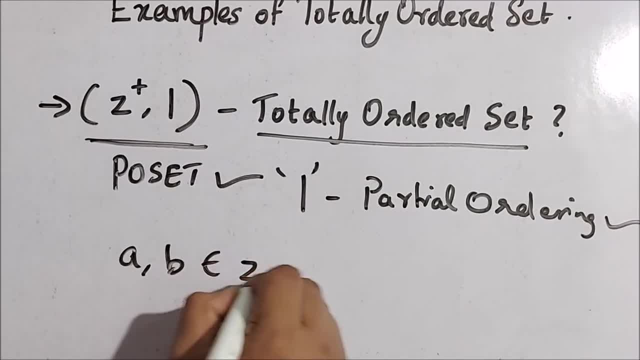 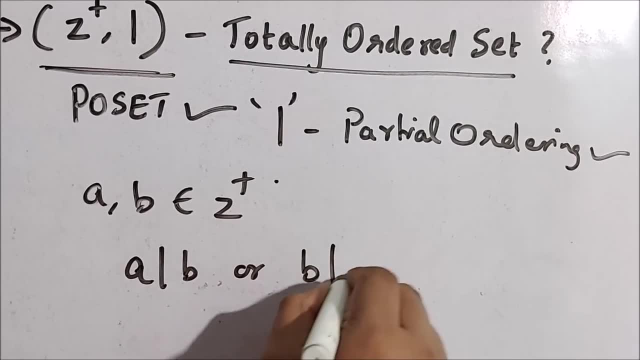 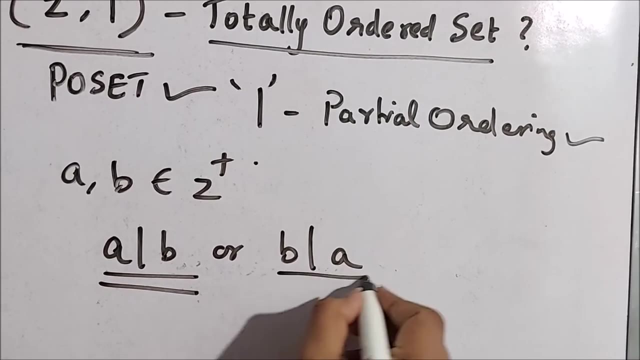 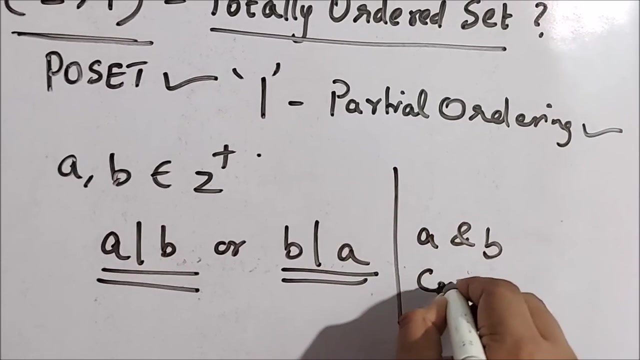 So you take A comma B belonging to set plus any A comma B belonging to set plus, whether A is related to B or B is related to A. So either it has to be the case that A is A divides B or it has to be the case that B divides A to say that A and B are comparable, Right. So what do you think? 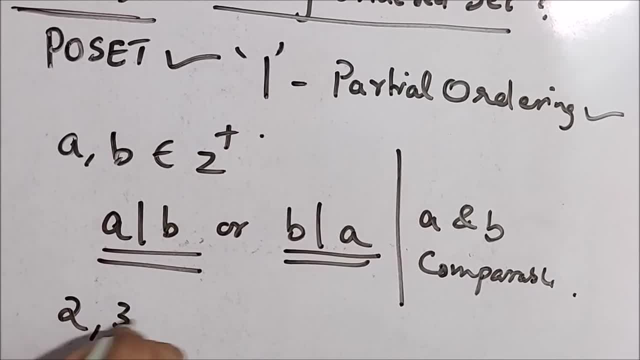 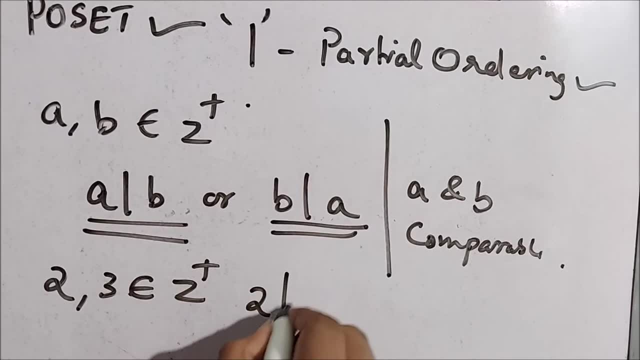 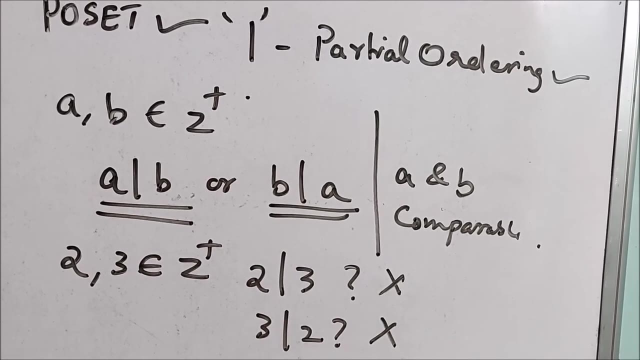 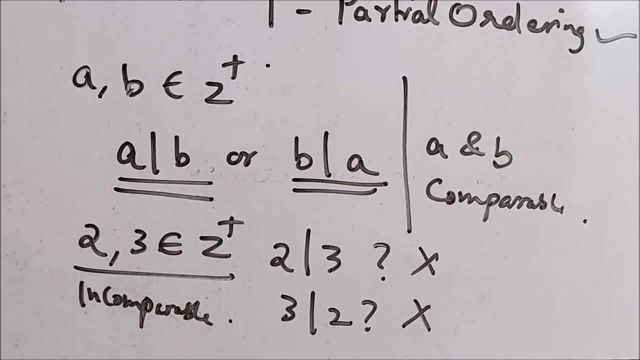 Okay, Let's take the elements 2 and 3.. Okay, 2 and 3, both are elements of set plus Right. But whether 2 divides 3? No Right. Whether 3 divides 2? No Right. And hence we have two elements which are incomparable, Right. And this is the reason why the set of positive integers, together with the divides relation, is not a totally ordered set, Right.